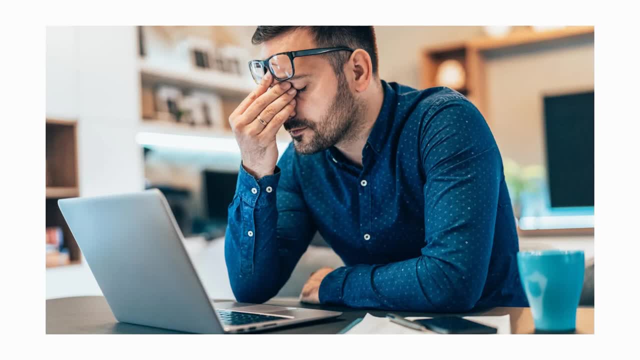 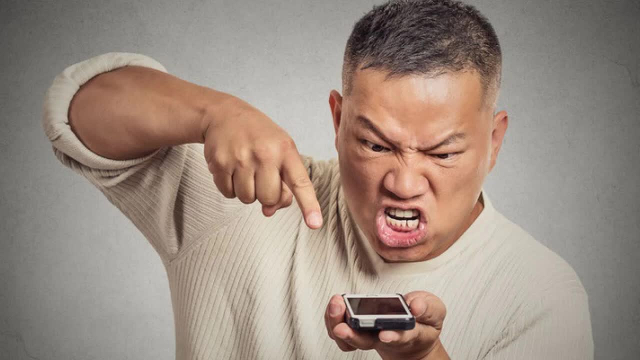 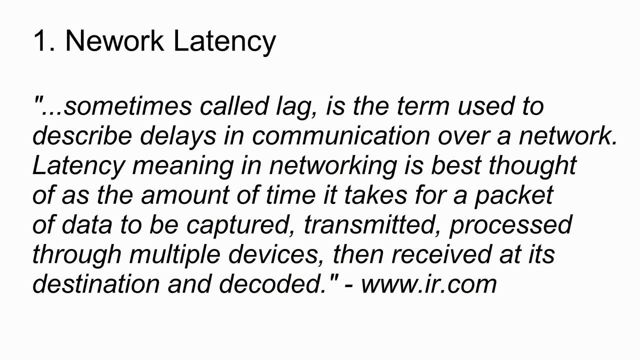 We take it for granted, when talking about network and network connections, what it actually means when you say the network is bad or the network performance is bad. So let's break it down into two major categories. The first would be network latency: the time it takes to get packets from point A to point B and then from point B back to point A. 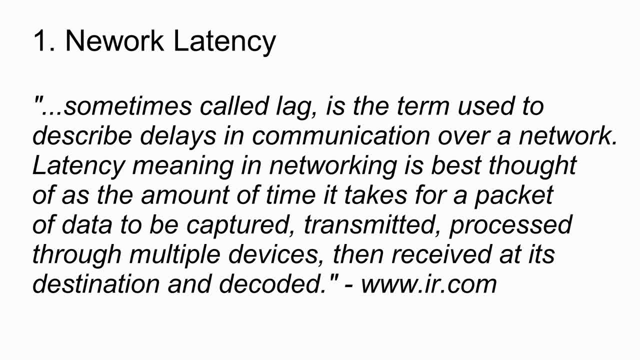 So latency is generally a function of the actual underlying physical network that connects the two. If it's within a LAN environment where you control the entire network generally speaking, the latency will be very stable, Whereas if you're routing over something like the public interface. 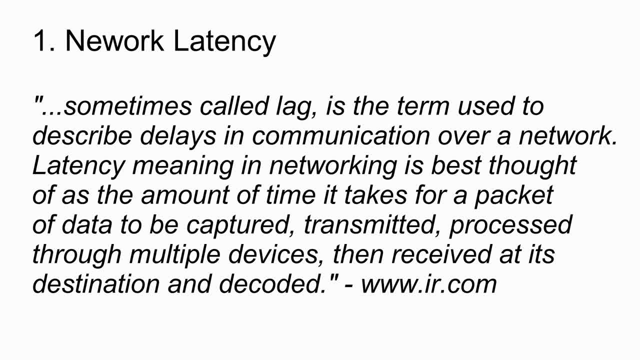 your latency might fluctuate quite a bit. There's also cases where devices that are intermediate to the connection, say a misbehaving switch or router, a load balancer, et cetera, can be inducing additional latency on some packets. That can have an effect on a connection, that's for sure. 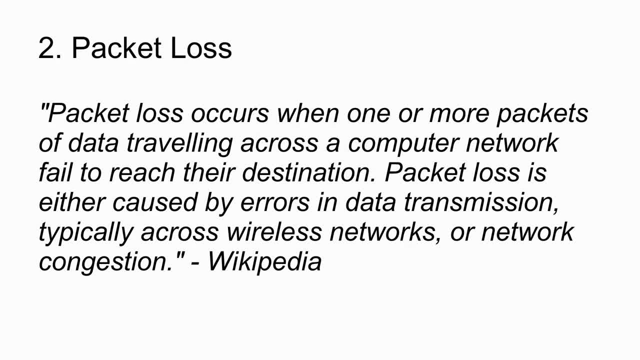 The second part is what happens when some of those messages between the client and server are lost, which is packet loss. This is also a common occurrence And it's generally pretty easy to spot in Wireshark. So we're going to go into both. 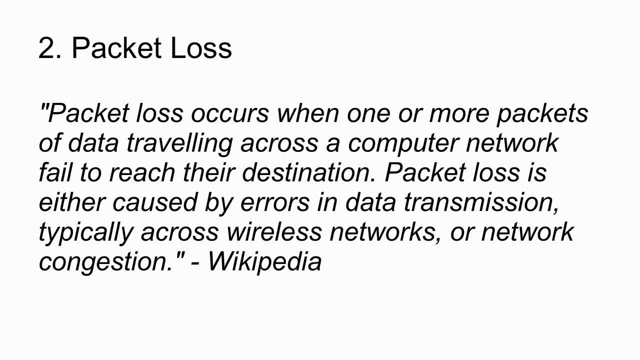 The first one we're going to dive into is the latency and actually how to pick apart application latency versus network latency. And then the second part is just quickly how to spot TCP retransmissions and packet loss in a connection, And if neither of those are an issue, you can be fairly safe in saying that any performance issue you're having is likely due to the application that's riding on the network. 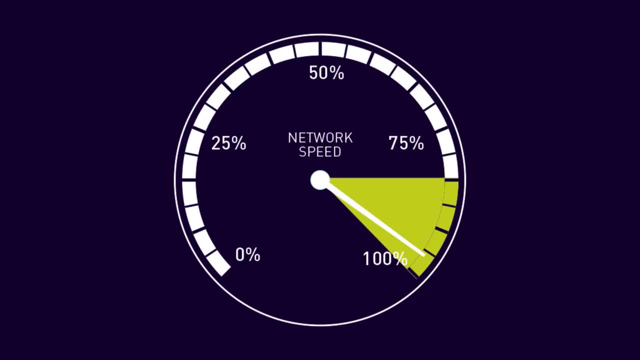 Now some of you may be asking: what about capacity? What if I max out all of the 100 megabit per second of my server's interface? Was that going to cause impact as well? And the answer is yes, it will. 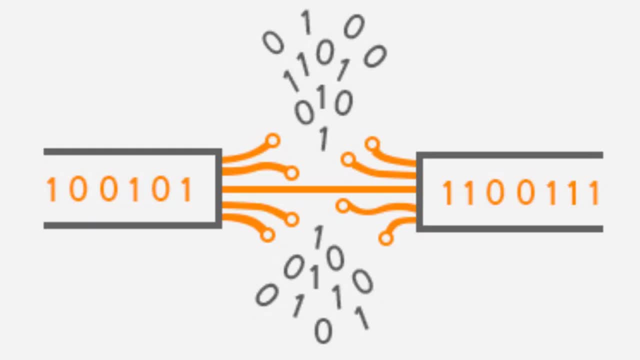 But that falls into the second category that we just discussed, which is retransmissions and packet loss. What will happen in TCP is that TCP naturally will try to fill up as much of the pipe as it can And when it actually gets to the point where it's. 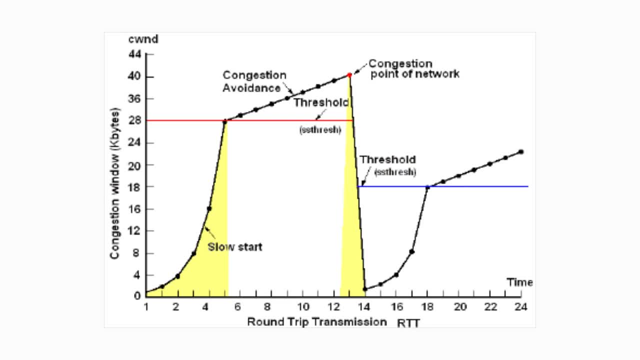 maxing out the total throughput of a given link, you'll actually start seeing some packet loss and you'll see retransmissions. So the analysis to actually spot retransmissions and packet loss also applies to conditions where you're hitting maximum capacity of a certain link. 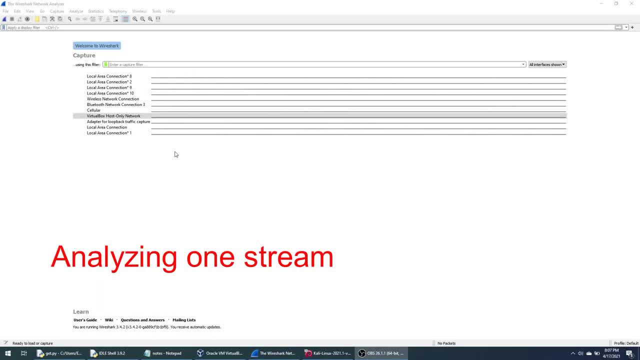 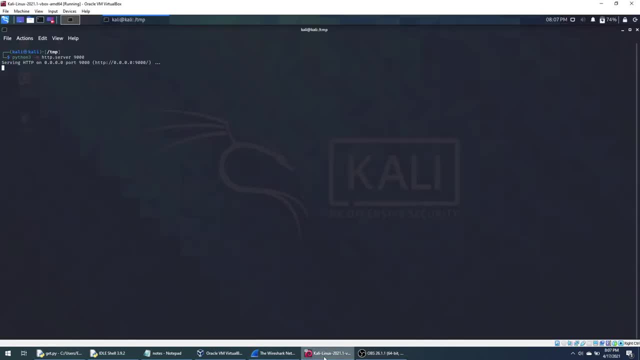 So for this example, I set up a quick testbed just locally here on my PC And what we have is a simple HTTP connection. So I've got a HTTP server running in a Linux VM- this is Kali Linux- and running an HTTP server on port 9000. 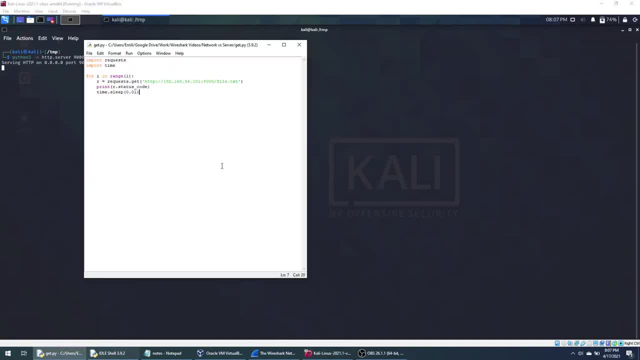 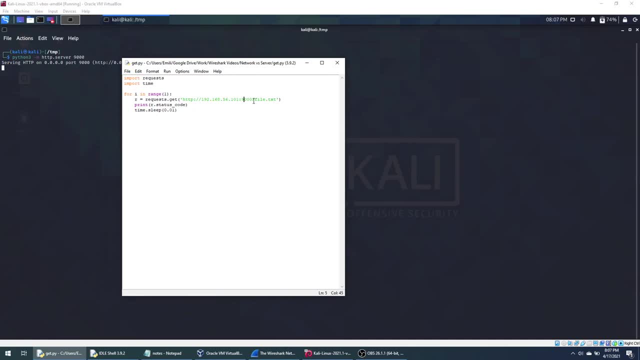 And at the same time, on my Windows machine I actually have a Python script which connects to that virtual machine on port 9000 and pulls down a simple file. Now, this is just a garbage file that I put onto the web server folder and it just contains random data. 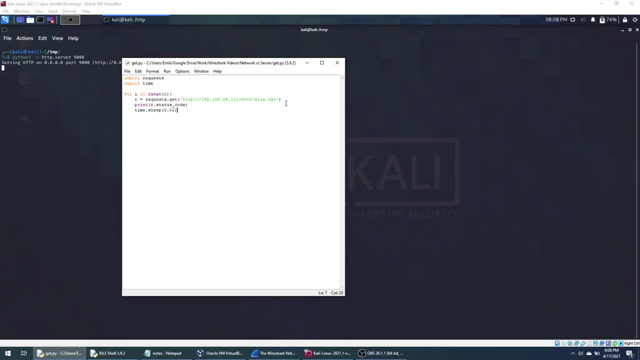 So the script will actually connect to the web server. It pulls the file, it prints the status code and then it sleeps for a period of time. In this case, for the first example, I've just set the number of iterations of the loop to one, so we can actually just see what it looks like. 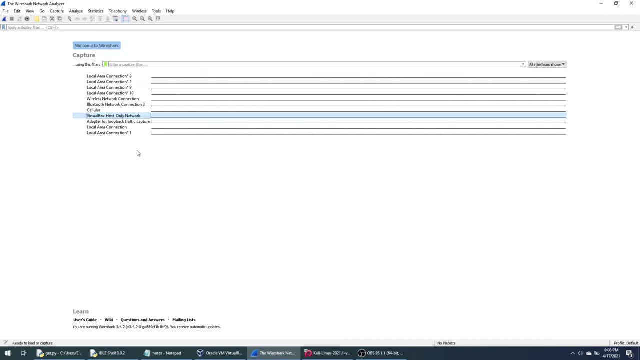 And then in Wireshark for VirtualBox, in order to capture this traffic. I've got the VirtualBox host-only network adapter selected, So let's do that. And then for the capture filter, just to keep things clean, I'm going to put port 9000.. 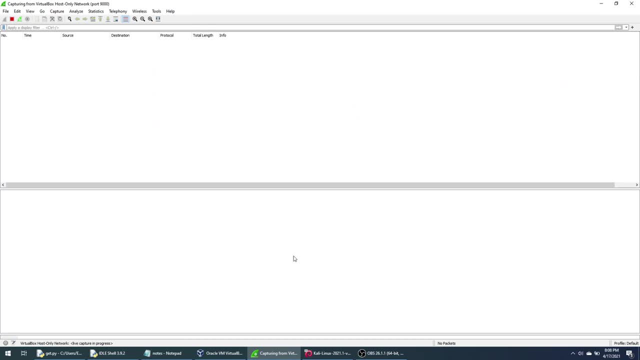 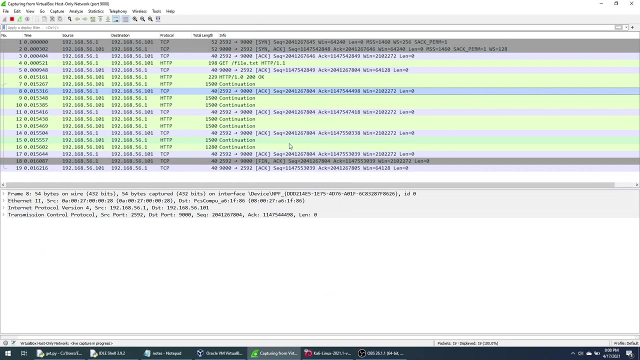 I'm going to hit start, So let's kick off the script And we can see we printed the status code of 200.. And to get started, let's just look at one HTTP request in Wireshark. So HTTP is a TCP protocol. 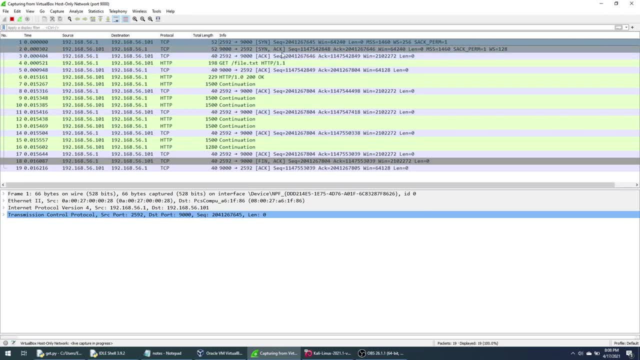 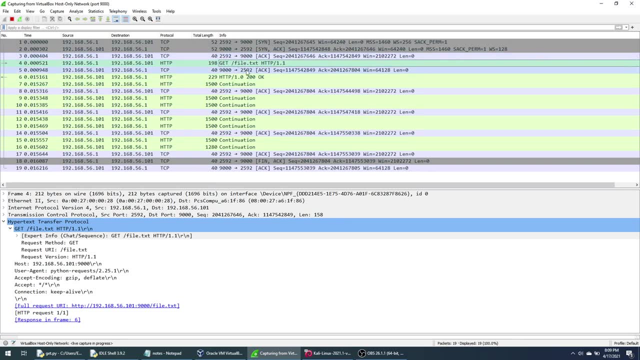 It runs on TCP. We have SINCENAC-AC Followed by a GET, So this is the first HTTP message: GET, file ITXT. That message is acknowledged And then we have HTTP 200- OK, meaning the web server acknowledges the request and is going to serve the data. 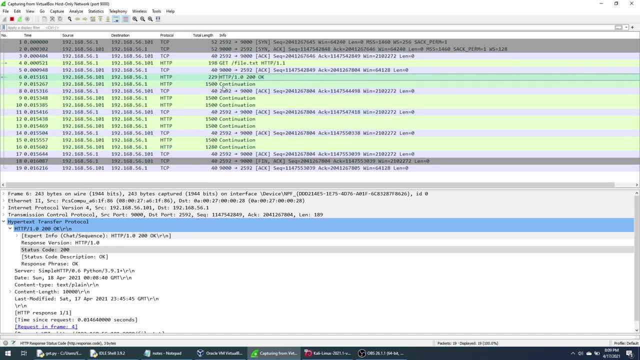 And then the remainder of the stream is dedicated to actually transferring that file. That file is something like 10,000 bytes And you can see here it's transferred in chunks And then at the end of the stream you've got a SINCENAC-AC. 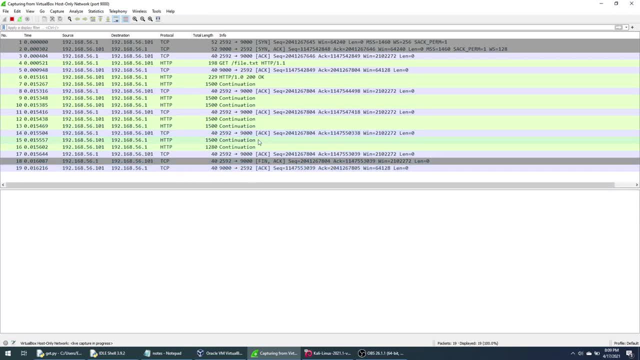 And then the actual conversation is closed. So it's pretty simple. Now there's a few things that we can dig into to actually pick apart the speed of the network and the transfer. I should say speed, I should say the transfer efficiency of the network versus that of the application. 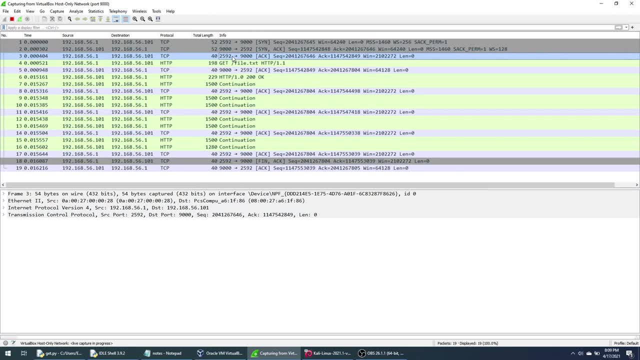 The first thing is to try to figure out what the round trip time of between the server and the client is, So to do that you can actually look at Some of the messages in the TCP stream other than application messages. So I mentioned this before. 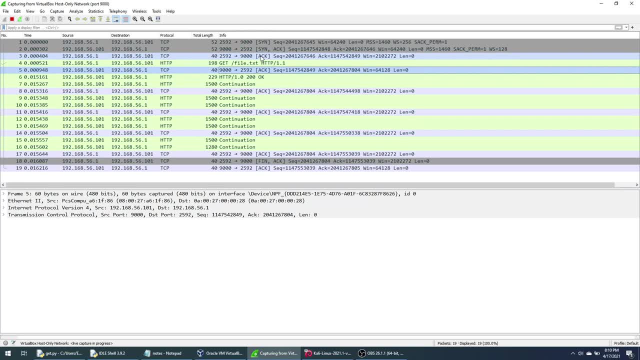 This. we consider this, for example, a naked acknowledgment, The acknowledgment in the three-way handshake. the final acknowledgment here, ACK. we call it naked because it really doesn't have any application data in it. It's really just a TCP control packet. 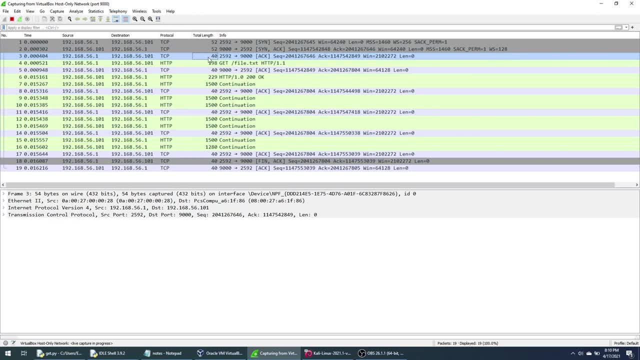 So this doesn't actually interact with the application layer. This is really just layer four in TCP. So we can use these messages to kind of get a sense of how, what the round trip time is between the client, the server and also how the actual network itself is performing versus the application. 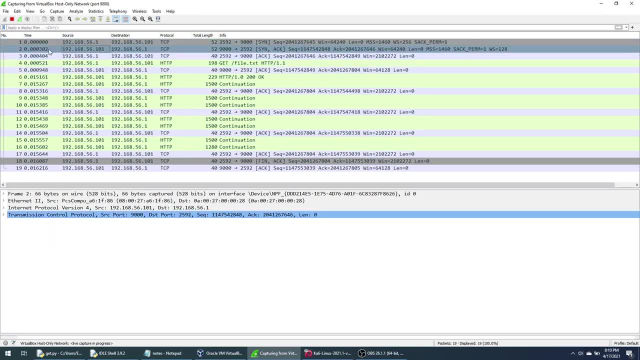 So if you want to take a look at the since an ACK- and we're going to look at the timings here now, these timings are in seconds. if you want, you can always change the time display format to make it easier for you to read, but you can. 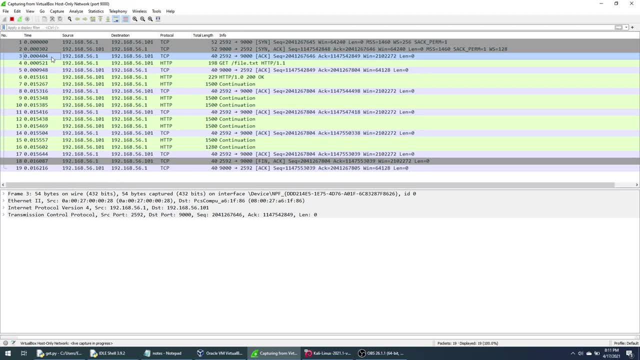 Follow along here with this example And then, if you do this on your own, you can actually play with the settings. So what you can see here is that the dot one machine, which is the client- that's my Windows machine- sends us in packet over to the server at time. reference zero. 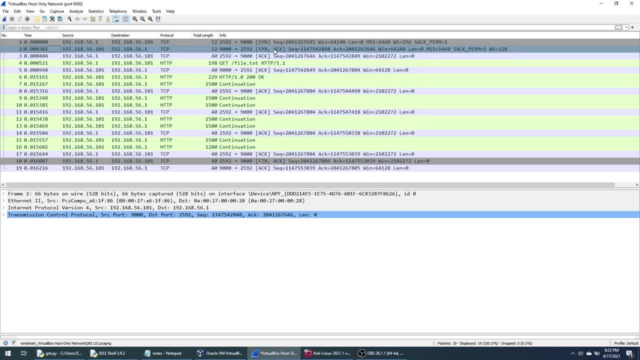 It takes point three milliseconds for that SIN ACK to get back to me, right? So that's from the server back to the client, to my Windows machine. And remember again, my Frame of reference where I'm capturing from is the client side. so I can roughly estimate that my round trip time between the client and server is about point three milliseconds. so that's important. 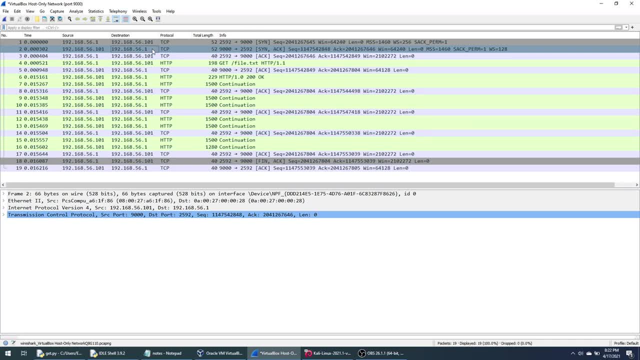 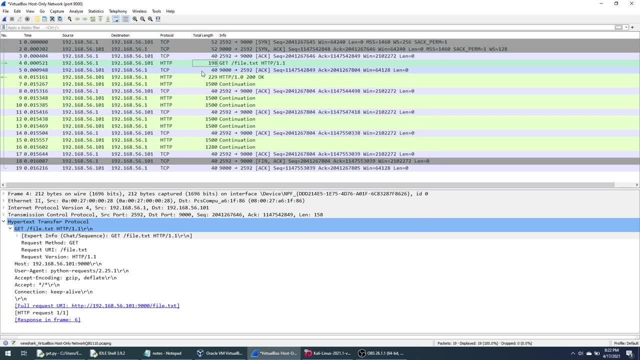 Keep that number in your mind. so my reference time, the actual time it takes to get a packet from A to B and back, is point three milliseconds. I can see that also reflected here in the get requests, So the get Request Request. 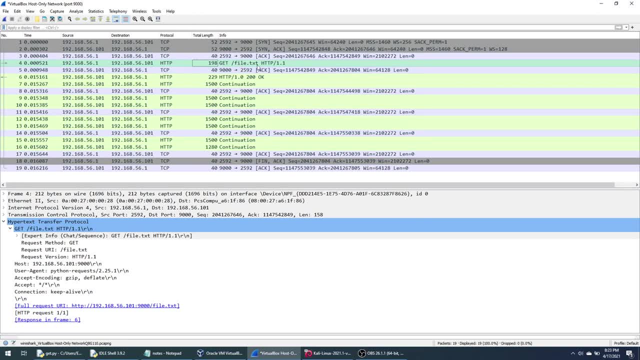 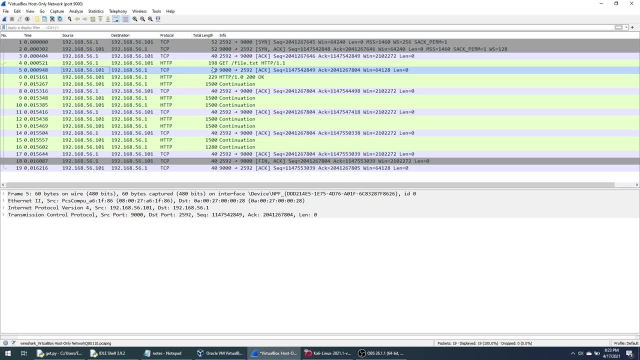 Request goes out. This is just a basic HTTP request. I send that to the server and now the server sends an acknowledgement back again in about- if I'm doing a quick math in my head and about point three milliseconds. If you want to actually get Wireshark to tell you what that is, you can actually go down to the TCP to sector. 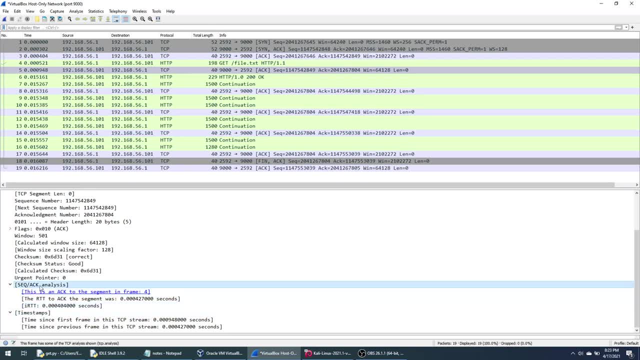 Open that up and then down here in a sequence acknowledgement analysis. it'll tell You what the round trip time is to act that segment. So in this case, again it's. it was about point four milliseconds. So in the first case it was point three milliseconds. 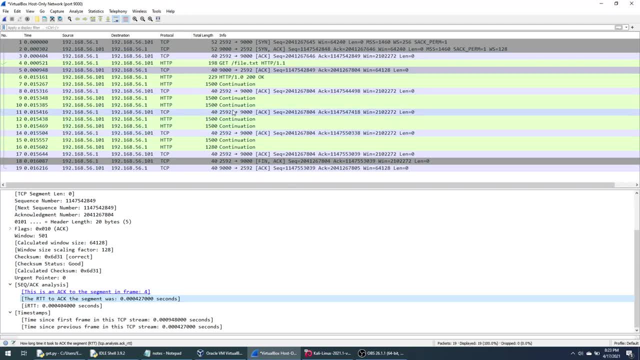 Here is point four milliseconds And as the stream goes on you can see that that hopefully, if this connection is stable, that round trip time will stay stable. Wireshark also has the ability to graph round trip time. I'm not going to get into that right here, but you can also Google that. 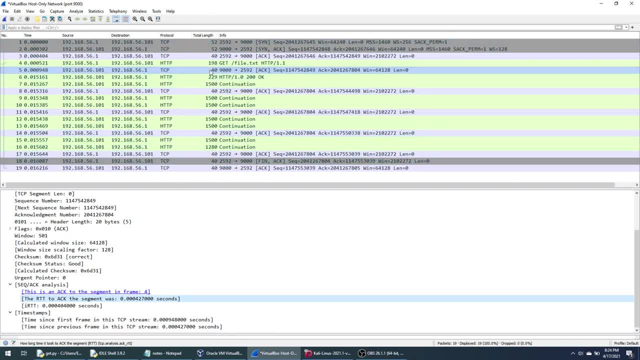 Look it up on YouTube So we know what the approximate time is to get a package from A to B. It's about point three to point four, milliseconds From there. we can then start looking at how long does it take, when I actually send that request to the server, for the server to return me data. 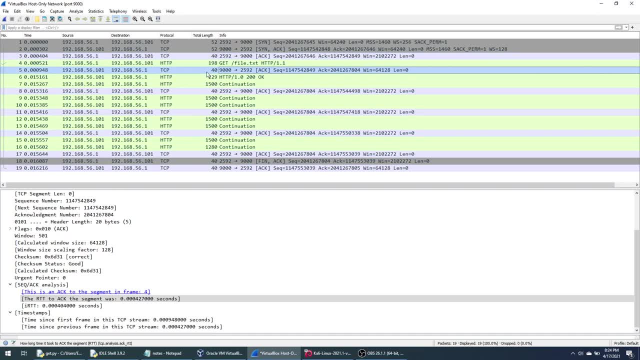 Because, remember, this acknowledgement is just saying: in TCP speak, I got your request. So, because it's a naked acknowledgement, it's not actually speaking HTTP. It's not saying: here is the file, that TXT file. It's just saying at the TCP layer, the server is telling the client: I got this packet here. 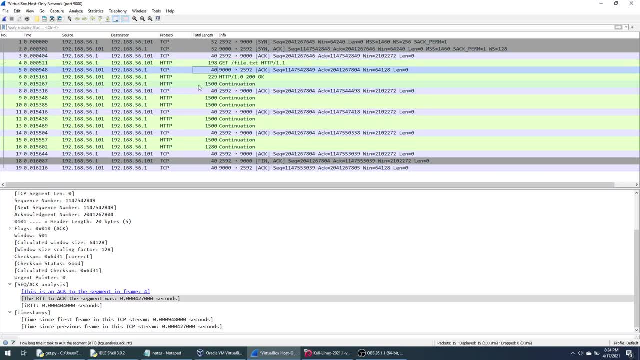 So what we need to know is how long it actually takes for the server to return the file that TXT request to the client. So if I actually look at the next packet down, this is 200. Okay. now in HTTP, 200 okay indicates that the request is all right and I'm going to start returning the data that you requested. 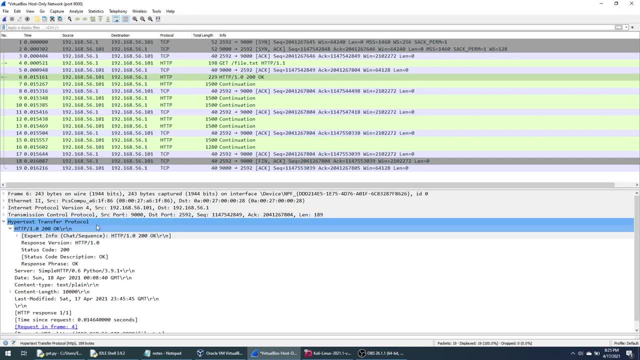 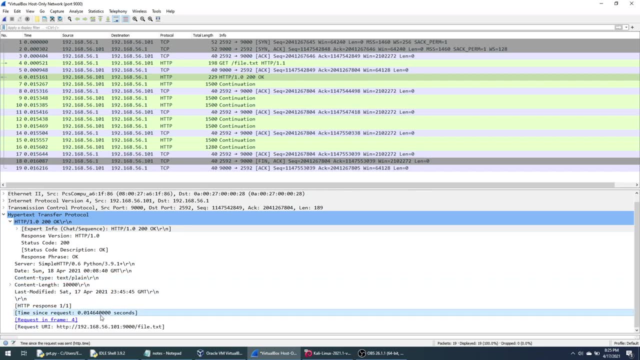 And if you wire struck again under the HTTP disector will tell you how long it actually took for the web server to return the to acknowledge the requests for that file to start the data transfer. So in here, for example, it says time, since the request is point 0146 seconds, so that's 14.6 milliseconds. 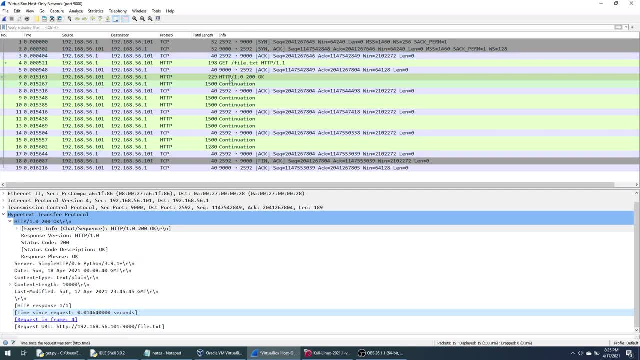 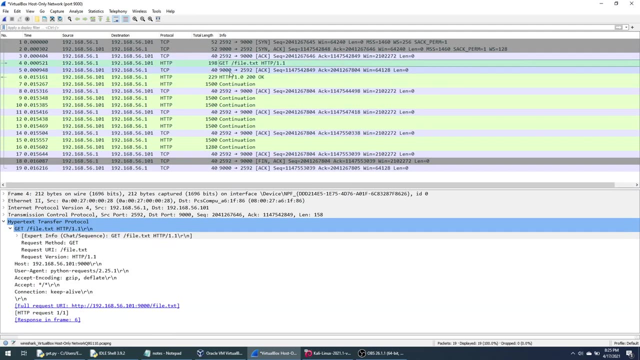 So let's look at those two numbers and keep them In your mind. it takes point four milliseconds to get a packet from A to B and back, But in this case it took 14 milliseconds from the time that that web server got there or time that we sent the request to the web server to the time that actually got us back with the 200. 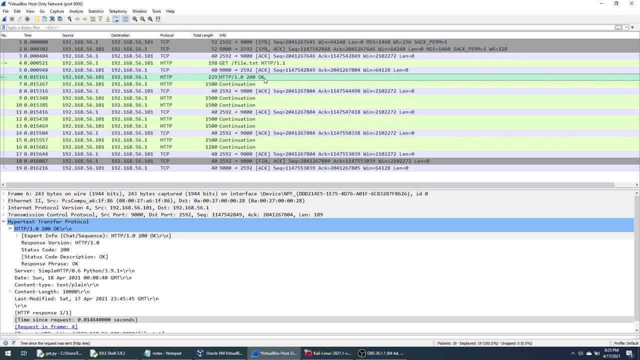 Okay, so this is a very small case And it's a microcosm of larger issues that can exist. But that's a very important distinction: How long it takes to get the packets from A to B and back, versus how long it takes for that web server to actually acknowledge the request and start sending application layer data back. 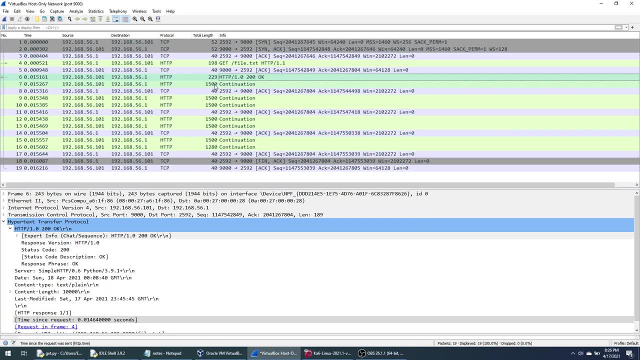 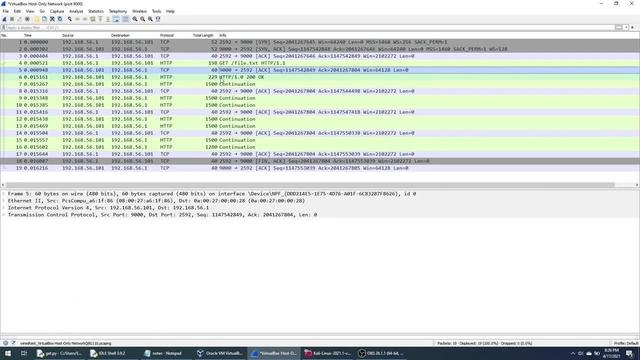 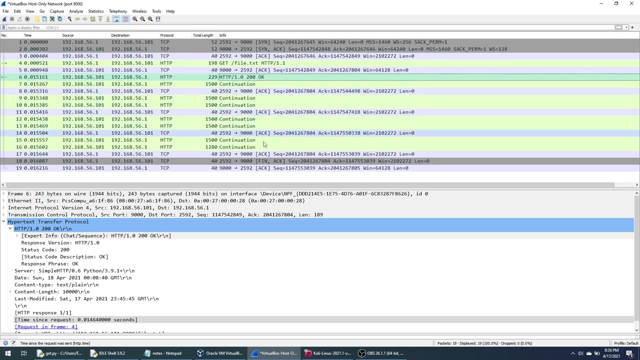 In this case. no one's going to complain about these speeds because these are all sub, sub, second, sub millisecond speeds, But you can see the difference. The network is able to get this acknowledgement packet back to the server, but it then takes an additional 14 milliseconds, 14.3 milliseconds, to return this 200 okay message to the client and then actually start transferring the data. 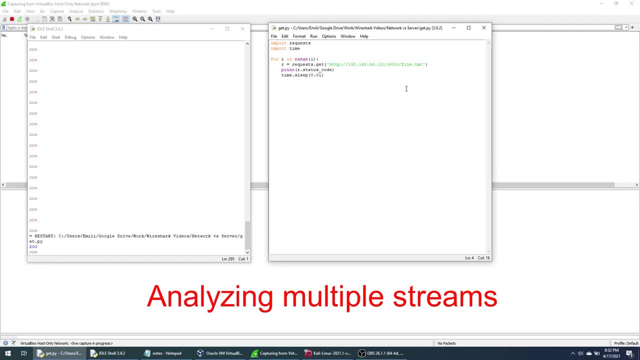 So the next thing I want to do is show you what this looks like at scale. So there's very few instances where someone will complain about one request going to a web server being slow. The typical example we get at work is API engineers, So either those who consume API resources or those who build APIs. 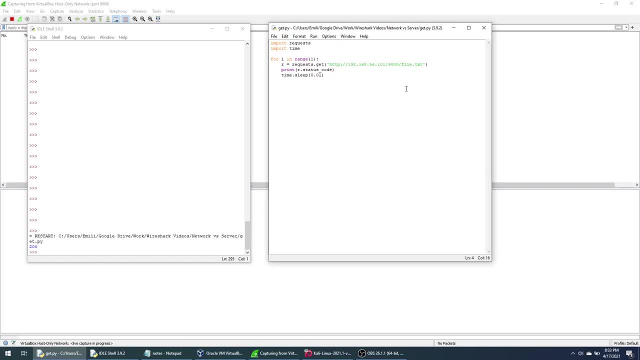 And with APIs it's generally HTTP protocol And it's you're talking about 10s, hundreds, thousands of transactions per second against these servers. So when performance issues happen, it's not good enough to just look at one request. You're not going to get there. You're going to lose this. You're not going to get there. You're going to lose this. You're not going to get there. You're not going to get there. So you're not going to get there. You're not going to get there. 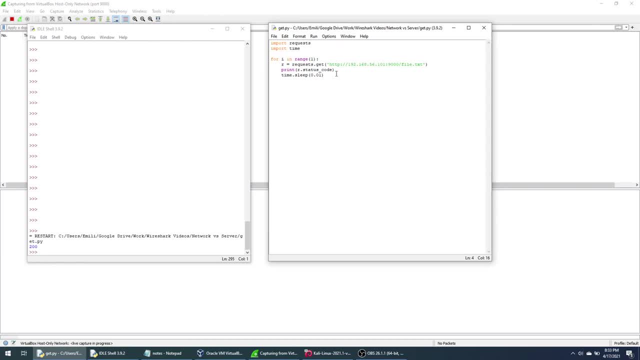 You kind of have to look at it with the macro view. So to do that, what we're going to do is actually in this simple Python script I'm going to turn this up to we're going to do about 40 requests. 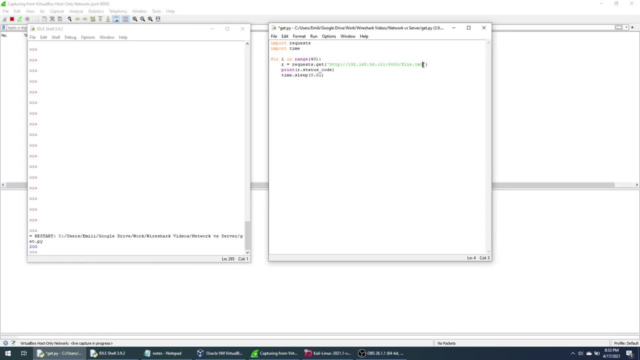 So what this loop will do is go through 40 times, connect, download the file, print the status code and then sleep for about- in this case it's 10 milliseconds, and then run the script again. Okay, so it's really just going to generate a lot of requests at once. 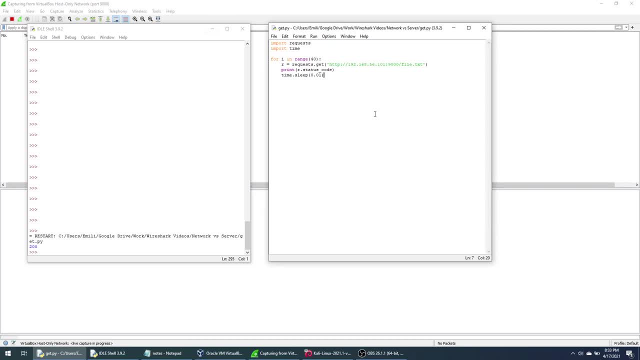 So I'm going to save that and then let's run it. And in the background in Wireshark I've got the same host or, sorry, same capture filter in port 9000.. So let's run that And you can see here all the 200, okays? 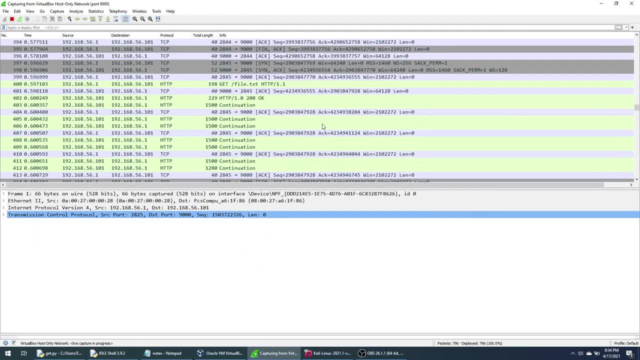 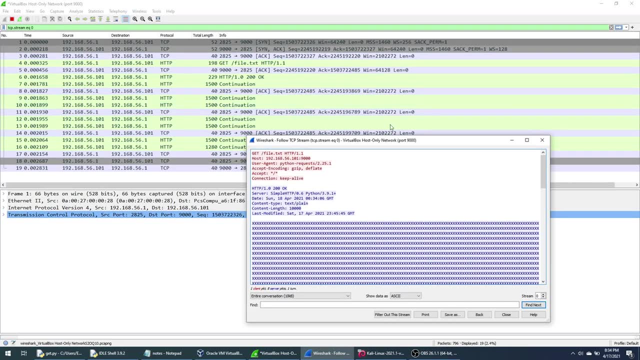 and you've got tons of data in Wireshark for all the requests, So we're just going to start with one. So let's go to the start, right-click, follow TCP stream. You can see here my text file is just a bunch of Xs. 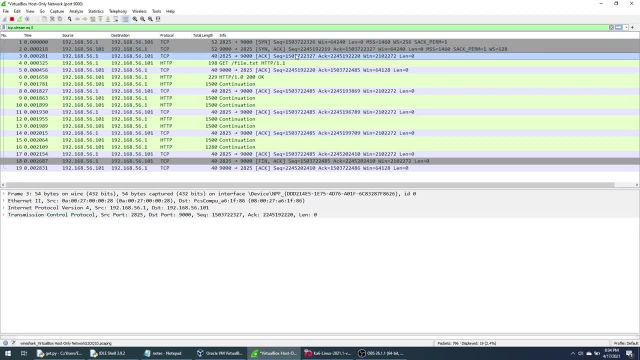 And we're going to do two things. We're going to look at the acknowledgement here. This is the one that we looked at previously to actually find and actually blah, Fuck, start again. So we're going to look at two things here. 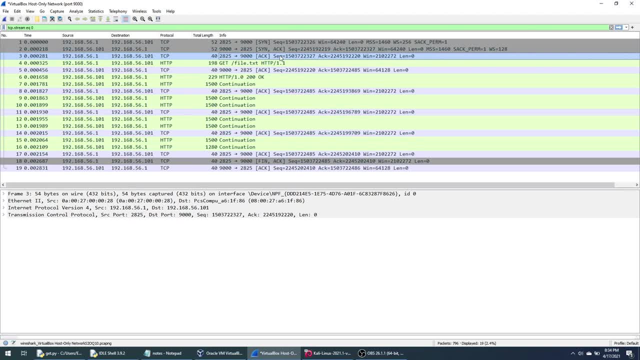 So, with this individual stream, I want to pick out two metrics that we can use to compare. The first one is the round-trip time of this SYNAC, which we looked at in the first example. Here you can see that it takes about 0.2 milliseconds to get this SYNAC back to me. 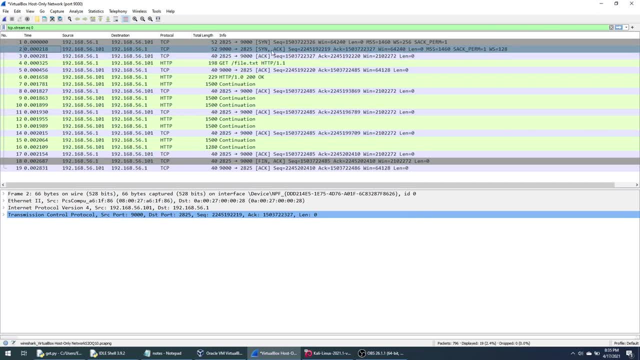 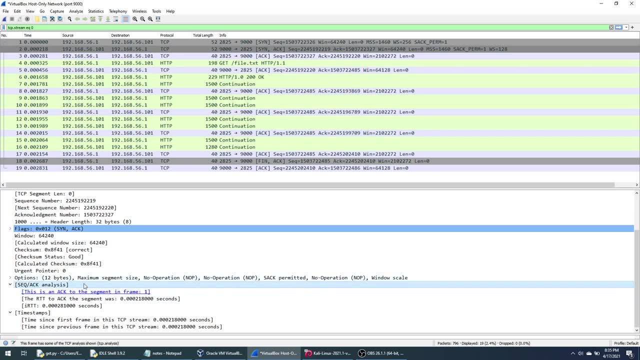 So I actually want to look at the round-trip time of this SYNAC and I actually want to have this as part of a filter. So the first thing I want to do is actually, in the TCP control protocol, go down to sequence acknowledgement analysis. 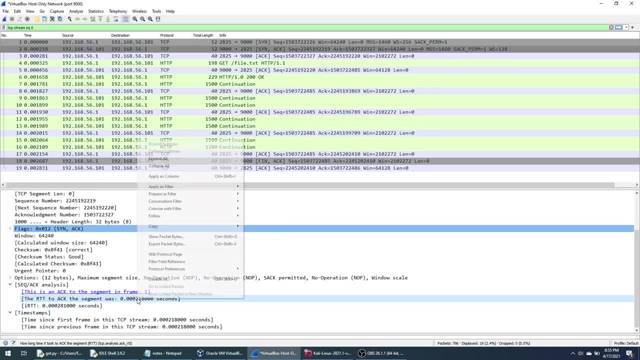 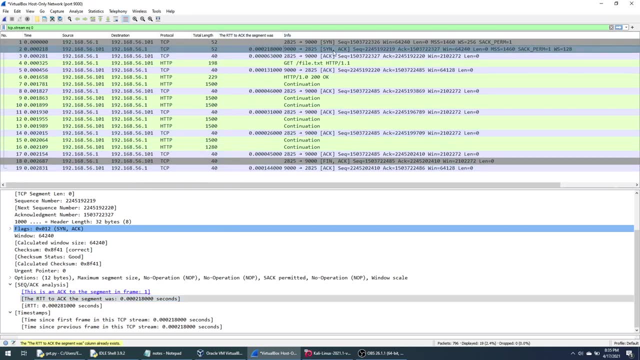 and then this calculation where it calculates RTT. I want to place that as a column, So the RTT active segment was this. And then I actually just want to look at SYNAC packets. So for that I can either build the filter. 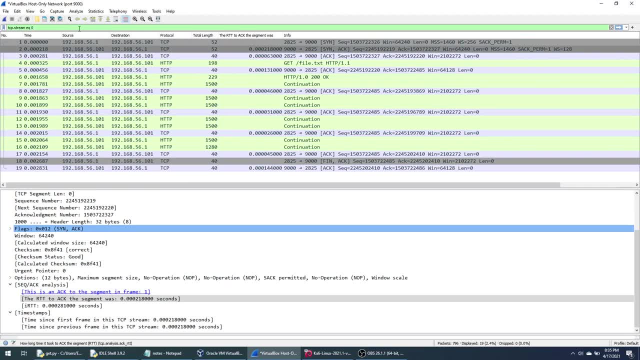 and actually you know what I probably will. That filter is going to be: tcpflagssyn is equal to 1, and tcpflagsac is equal to 1.. So I'm just going to save that for now, and we'll use it again next. 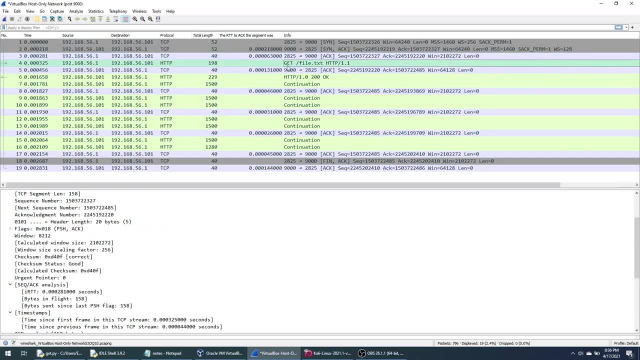 The next thing I want to look at is how long it takes the actual web server to return the 200 OK back to the client, And now we looked at that in the previous example. again, Wireshark will have a nice dissector for that down here. 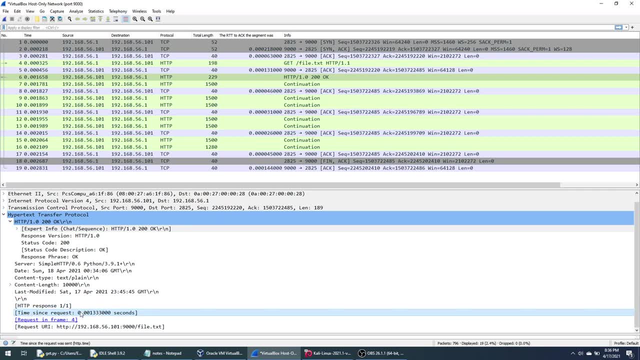 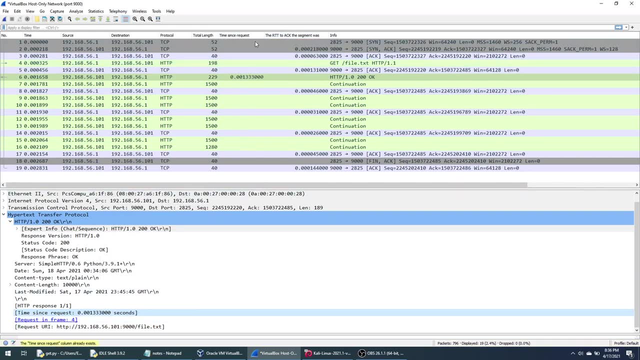 TimeSenseRequest. So this is TimeSense HTTP request versus here. this is the round trip time of the actual ACK packet, So let's apply this as a column as well And just remember the difference between the two. This one is the SYNAC packet- RTT. 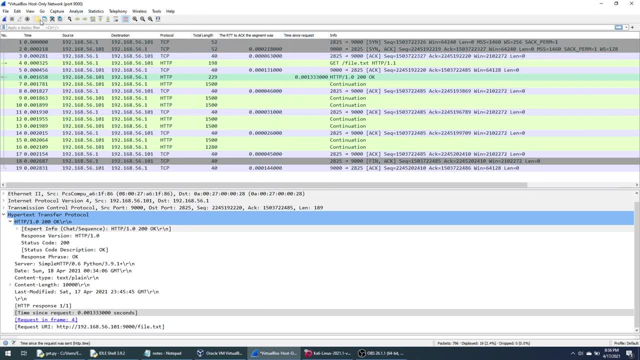 and this one is the HTTP TimeSenseRequest And I'm going to build the filter. I'm going to say I want to look at packets that are SYNACs. So the SYN flag is 1 and the ACK flag is 1.. 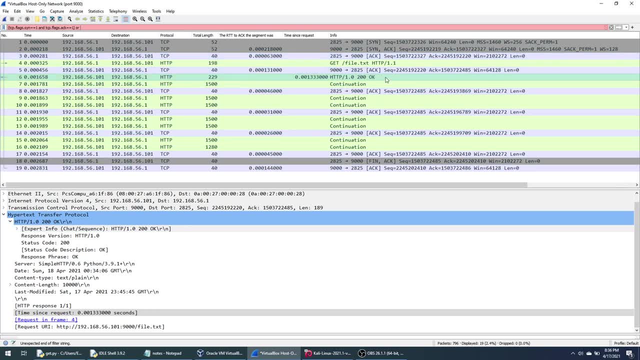 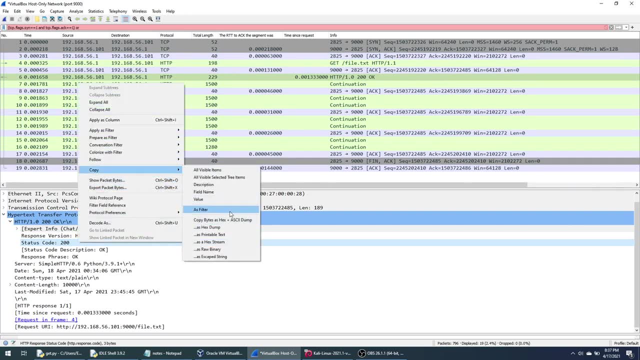 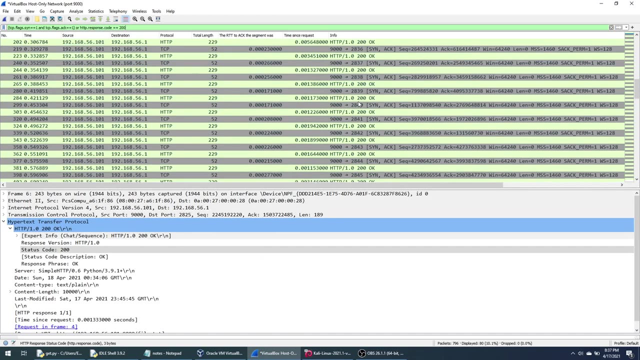 Or I want to look at 200 OKs. So what I'm going to do is actually come over here to status code 200, right click, copy as filter and paste it up here, And I get something that looks like this: So let's talk about how to interpret this. 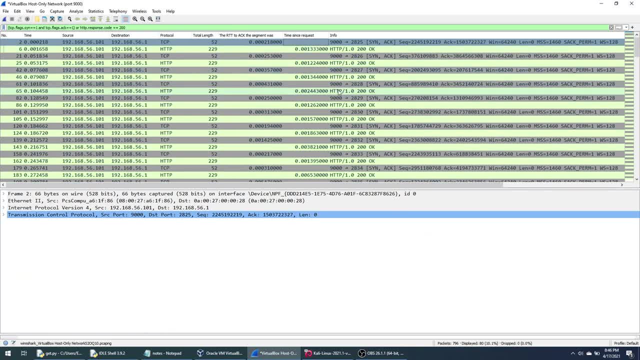 You can see here that this is encompassing all of the 40 or so TCP streams and HTTP requests that we made to the server. You can see here the time it takes to actually get that SYNAC back, which is roughly a measure of the round trip time. 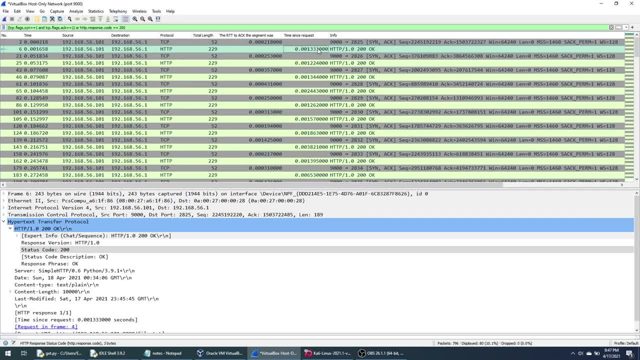 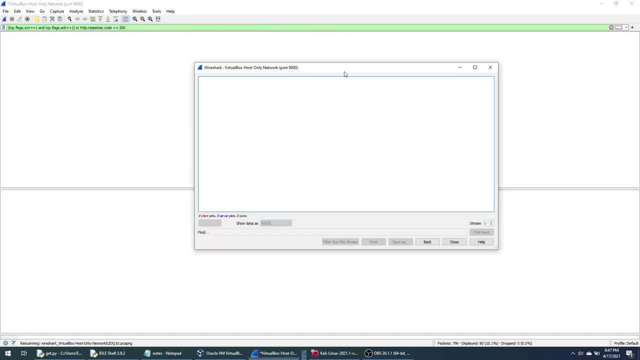 And then the time it takes for the server to return the HTTP 200. OK, So if I were just to look at the first, let's just copy this filter out for a sec. I want to look at the first stream. You can see here that this is the pass. 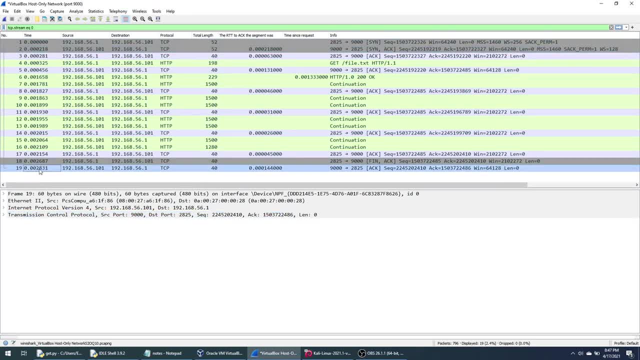 here that overall it takes about 2.8 milliseconds for this whole thing to finish. say, in your world that's 2.8 seconds and you're trying to figure out whether or not. okay, this is the client. you're trying to figure out whether this is the http server that's slow or it's network that's slow. 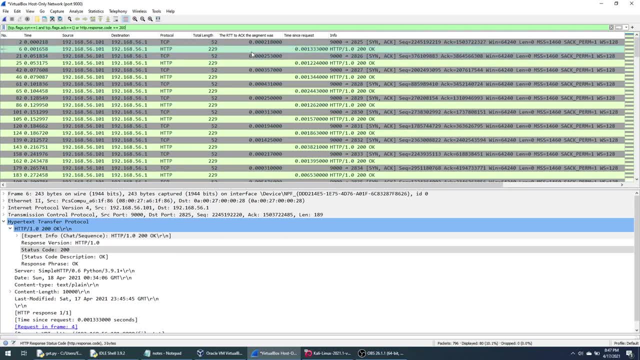 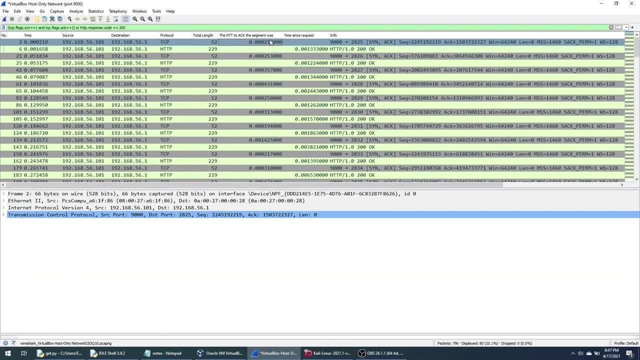 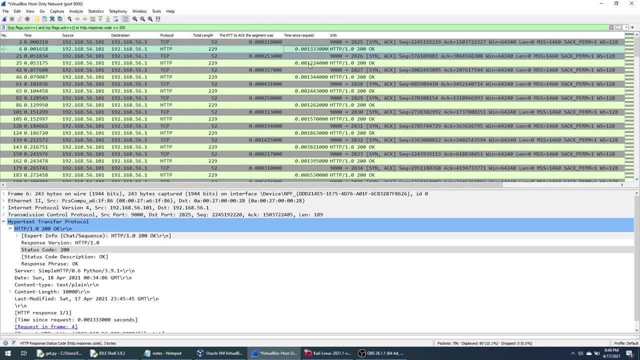 let's go back to the filter. with this on here, what this is telling you is that it takes roughly 0.3, 0.4- in this case 0.2- milliseconds to get packets from a to b, but it's actually taking the web server about one millisecond. 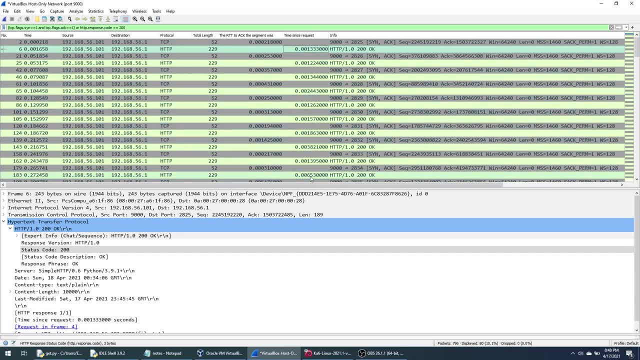 two milliseconds upwards of four milliseconds, six milliseconds to return the 200k back to the client. so if you're looking at the total duration of that session, more of the time is spent actually waiting for the server than it is and actually transporting the packets back forth. so this is a quick way of you looking at this at scale, this capture in front of us here. 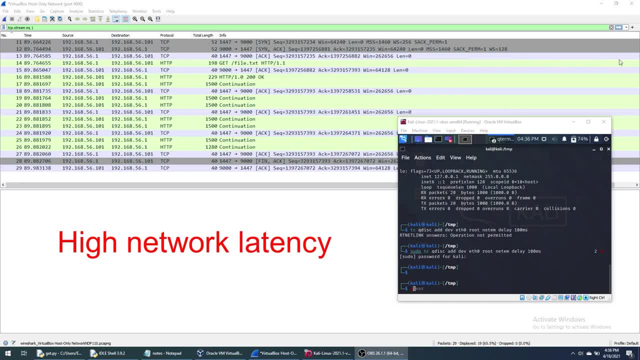 is a different scenario. what I did was in Kali Linux, there is a tool called tc which allows you to actually simulate both latency and packet loss on a given interface. so in the absence of actually machine that is 100 milliseconds away in terms of latency, we can simulate it using TC. So what? 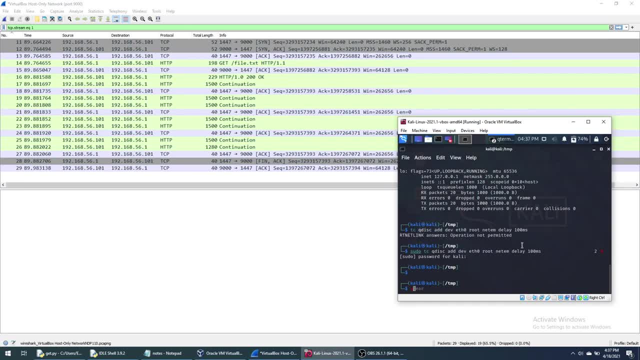 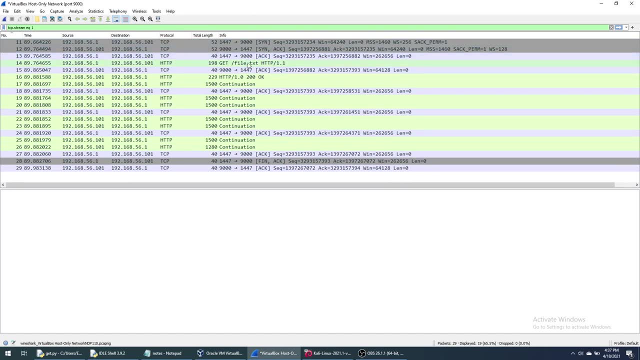 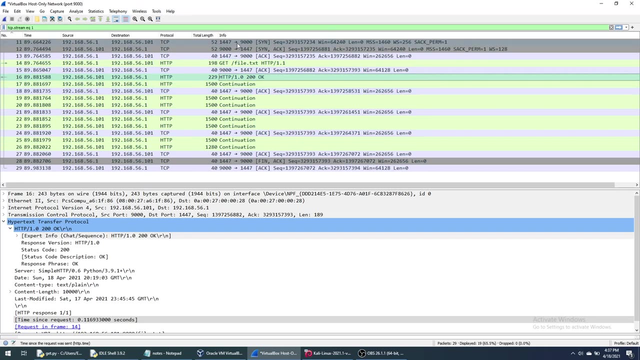 I've done is actually added 100 milliseconds of latency to the interface ETH0 of my virtual machine, And here in Wireshark is the actual capture of the same file transfer on port 9000, but it is with 100 milliseconds of latency. So let's look at the actual timings here. 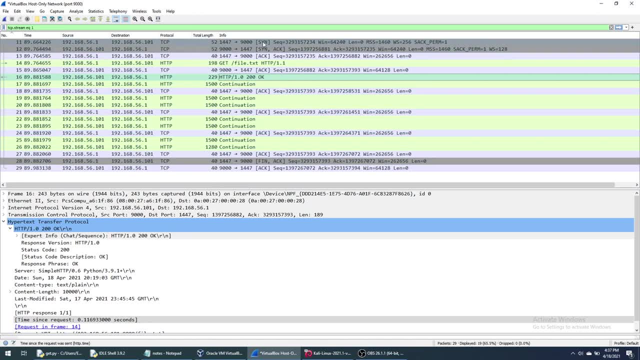 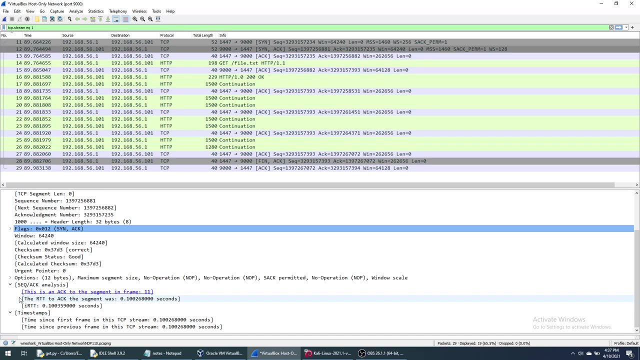 We see here that the SYN goes out. Again, we're the source of the capture. This is the Windows machine and dot one is the Windows machine. The SYNAC comes back Now. let's look at the timing here. If I go into TCP, you can see here that the RTT to active segment was 100 milliseconds. 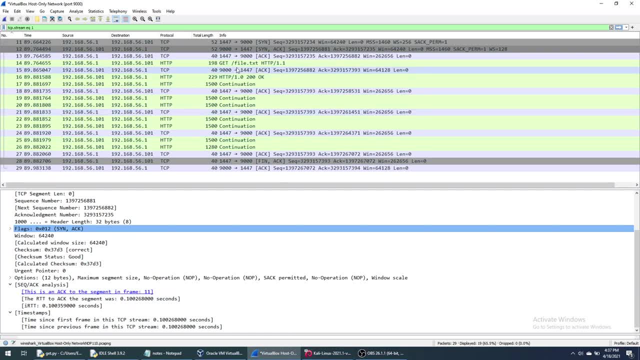 which is what we expect, because that's what I set in Kali. So the round trip time here is actually quite substantial relative to what it was before. So I'm going to go into TCP and I'm going to go into IPv4, which is actually just a fraction of a millisecond. Now let's look at the timing of the. 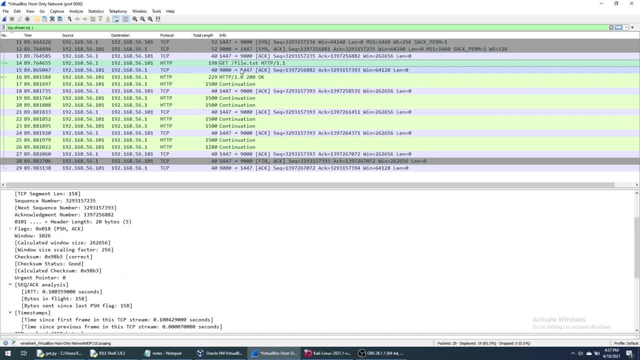 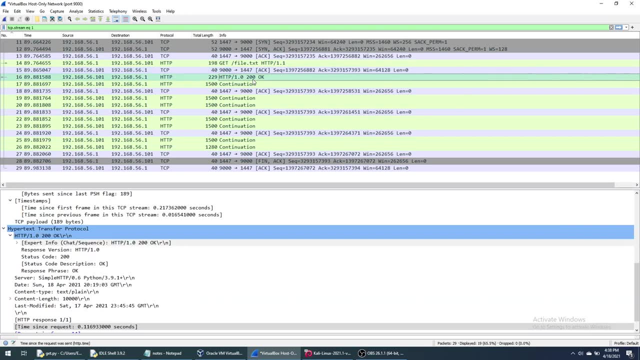 application layer messages. So the GET goes out. It's acknowledged again about 100 milliseconds. So the server got it. I acknowledged it And then the 200.. Okay, from the server comes in at about 116 milliseconds from the time that the GET went. got to the server Actually. 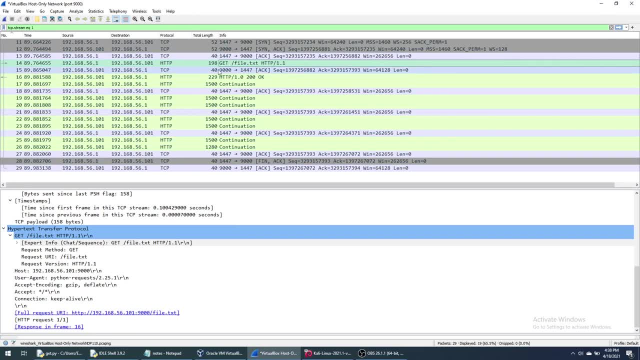 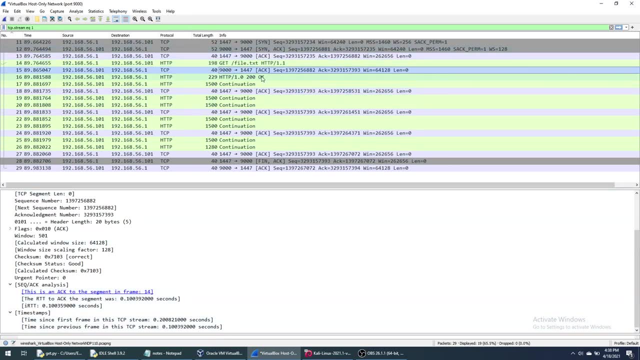 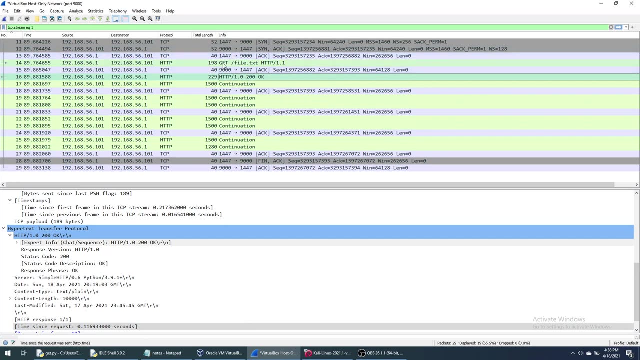 the same thing is true of the RTT. The GET goes out, but then it is at about 116 milliseconds. So the GET goes out, it's acknowledged in about 100 milliseconds, And then the 200.. Okay, comes back. then 200k comes back 116 milliseconds since the request was sent. So if you think about that, 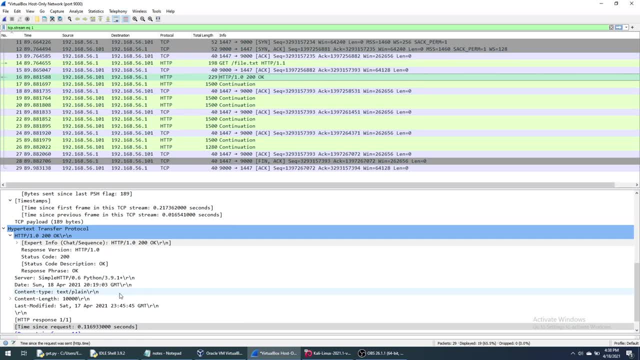 the overall round trip time in terms of the packet getting from A to B and back is 100 milliseconds, 16 milliseconds to return the 200 okay. So what that would apply is that it actually took the server about 16 milliseconds to do the processing, to get the 200 okay message and send it out. 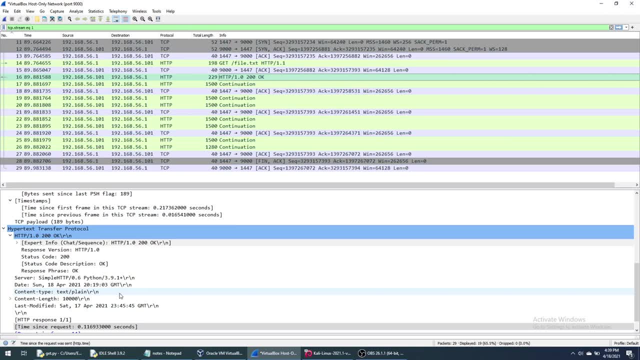 But it took 100 milliseconds on top of that to get the message from the server back to the client. So in this situation, network latency certainly has a strong effect on the connection speed. You would normally spot this the first time you run this connection. 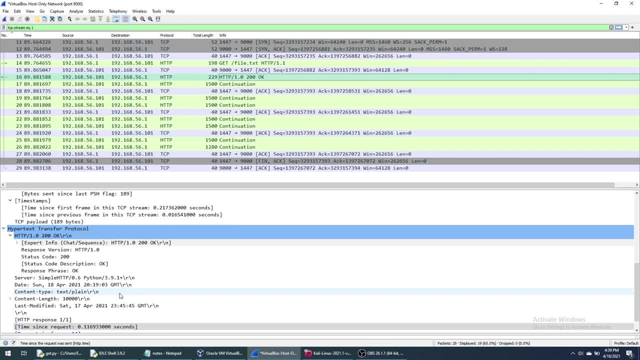 the latency of a given connection from A to B within, say, a private network, generally doesn't go up and down that much unless there's a problem. So if, for example, your API timing was X and then all of a sudden one day it's, you know, 2x, 3x in terms of the total time it takes. 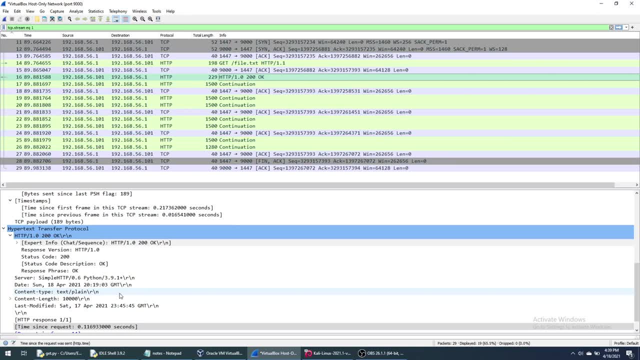 you may want to inspect to see whether or not the route has changed from the client to the server, If you're going over, when, for example, you're running a 10x connection, if somehow the carrier has flipped you to a protect path or something to that nature and then all of a sudden the latency is higher. because in these 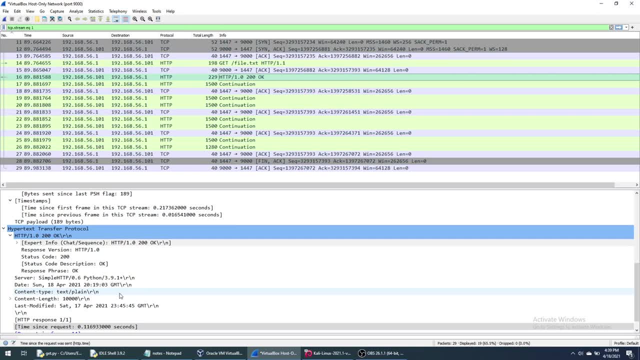 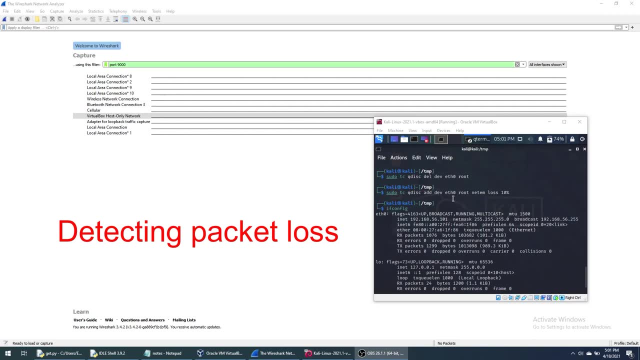 scenarios you can see, the latency actually would have a strong effect on the quality of the connection and the speed of the connection. Last example I want to cover is the example of packet loss. So how to detect packet loss in a Wireshark capture that may be affecting the performance of. 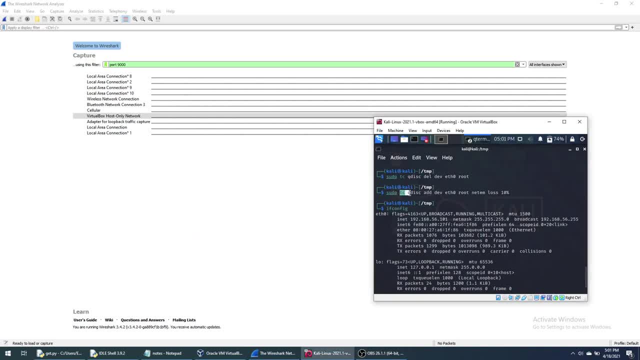 an application. So to do this again with the TC command, we've actually added the loss command of 10%. So what this will do is basically artificially drop one out of every 10 packets or 10%. So it's a good way to simulate packet loss. 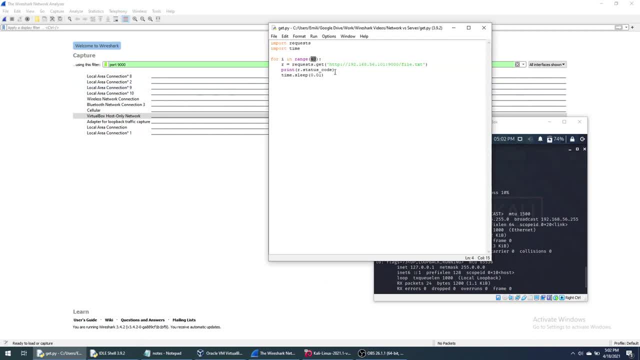 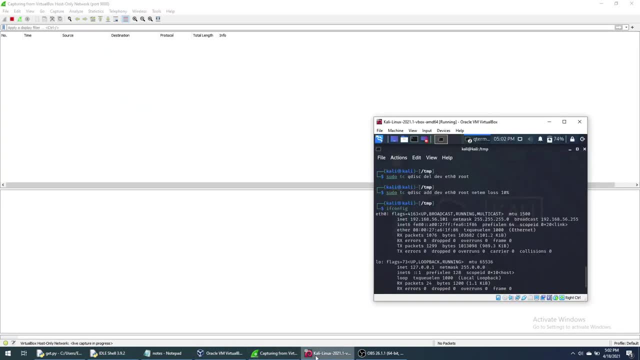 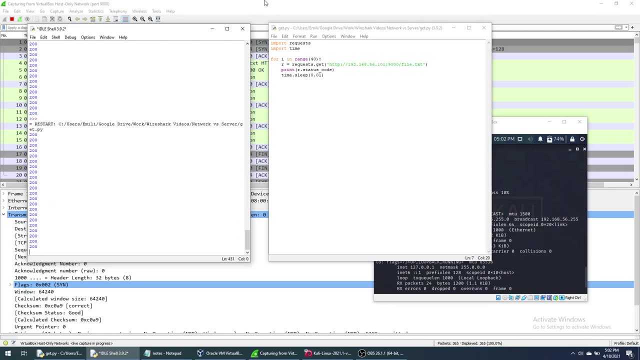 What we're going to do is actually take the script again, run it for 40 iterations and see what happens. So let's start our capture in Wireshark, port 9000. And kick off the script And you can see that it's doing the Wireshark report report. Let's see if we can start. 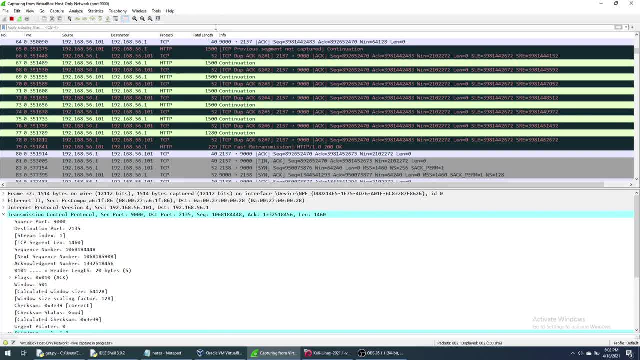 Let's take a look at what it looks like. So right away you can actually see wire shark has flagged some of these packets in block And you can see it actually has described this retransmission For the purpose of this video. I'm not going to go into sequence, acknowledgement, analysis and how to. 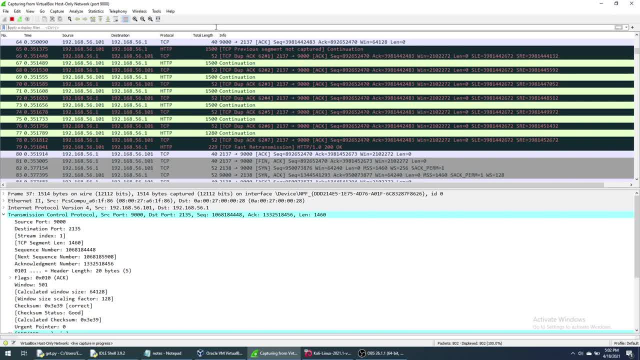 what you just need to be able to determine is: are there retransmissions within this capture? Wireshark has an easy way of doing that. You can apply the filter tcpanalysisretransmission and it'll show you all the packets that have been retransmitted within the capture. 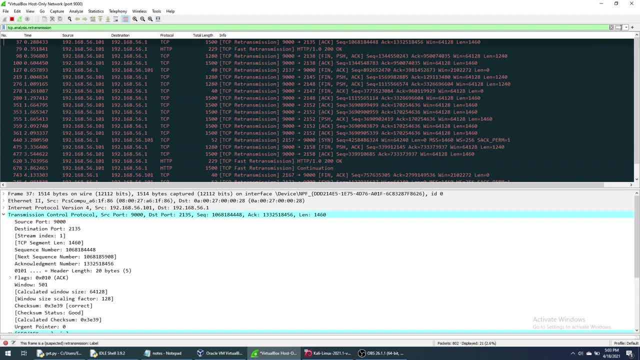 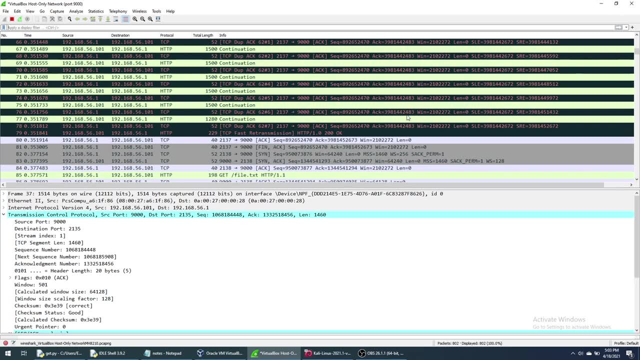 In this scenario I would say packet loss on the network can actually be a contributing factor to the slowness of the application. Anytime there is packet loss it requires additional time to catch up with that stream, so that lost packet has to actually be retransmitted. 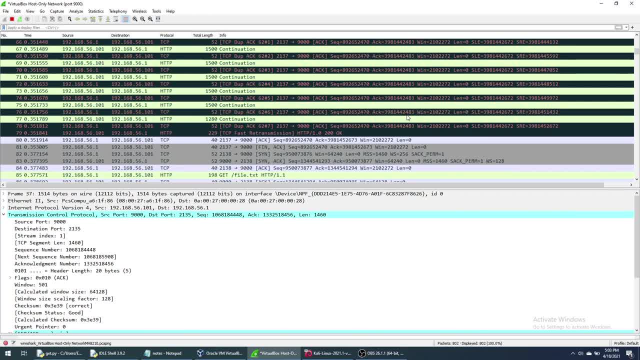 eventually from client to server, server to client and there's a lag time to actually get to that point where it's retransmitted. So that will certainly have impact on performance. However, if you do take the capture and you apply that filter and you see no evidence of retransmissions, 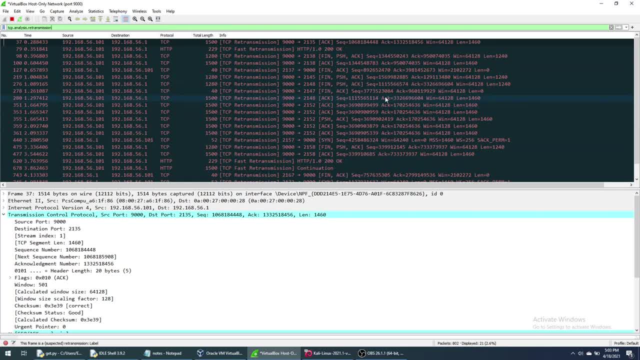 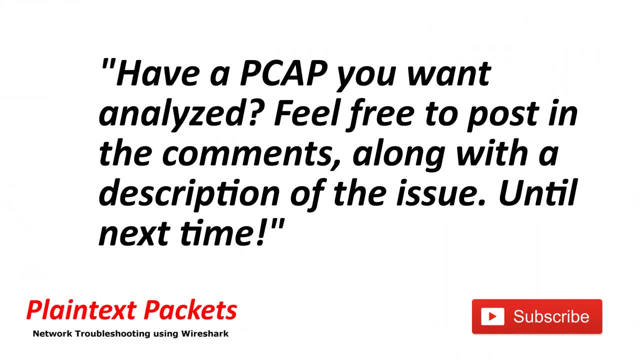 whatsoever, then you can be fairly certain that there was no packet loss in the capture. So that's it for today. The topic of tcp performance analysis is extremely lengthy. There's a lot of detail that we can go into and hopefully in future videos we can pick apart some of these topics in detail.